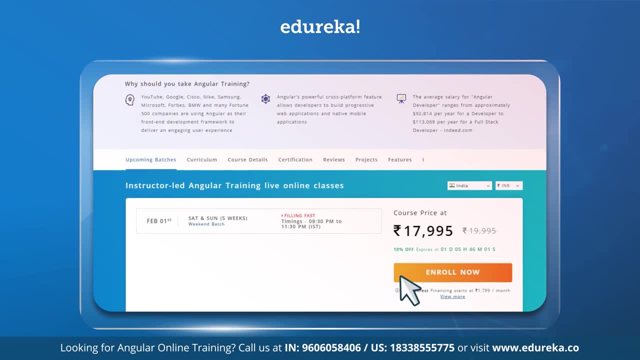 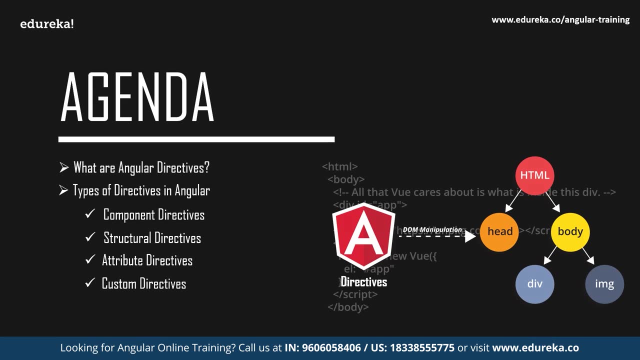 videos. Also, if you are interested in getting an online training certification in Angular, check out the link given in the description box below. Okay, so, without any further delays, let's move on. So what exactly are Angular directives? Angular directives are basically: 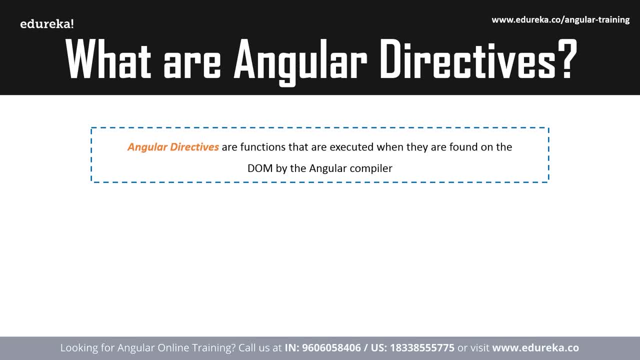 functions that are executed whenever they are discovered on the DOM by the Angular compiler. These directives empower the application's HTML through an advanced syntax. They have distinct names that can either be predefined by Angular or custom names defined by the user itself. A directive class in Angular is defined using the Etherate directive decorator. 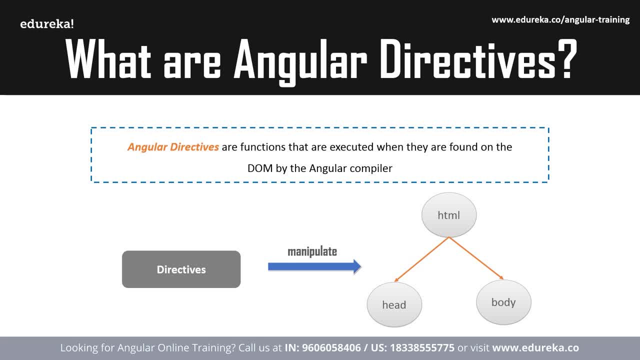 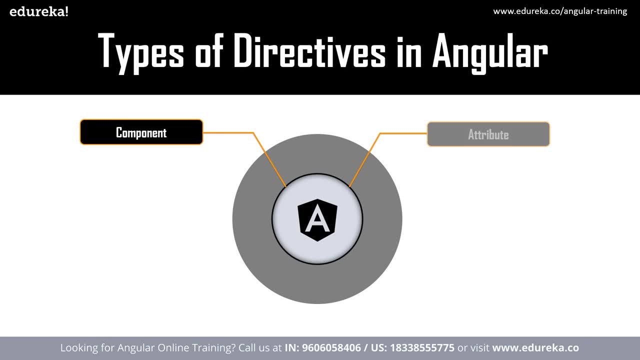 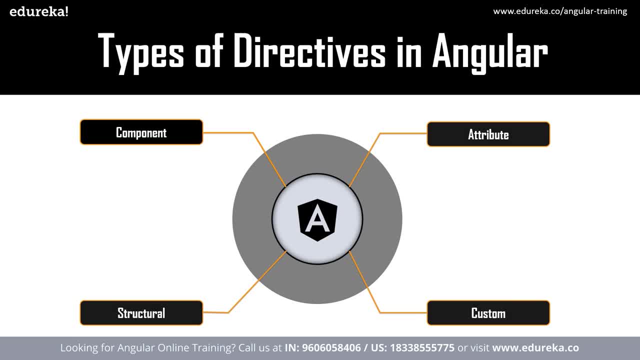 the structural directives, attribute directives and the custom directives, Components are nothing but a type of directives. The reason why they are defined specially under the Etherate component decorator is that components are very much distinctive and central to Angular. Factually, the Etherate component decorator actually extends the Etherate directive decorator. 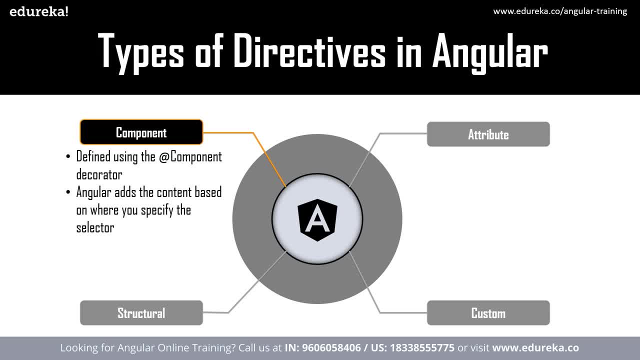 with features that are template-oriented. Whenever you add the selector of the component in the templates, you basically instruct Angular to add all the columns of the component design on top of it. every time it does something If you want to implement Tac, Laurent and Cartou치. 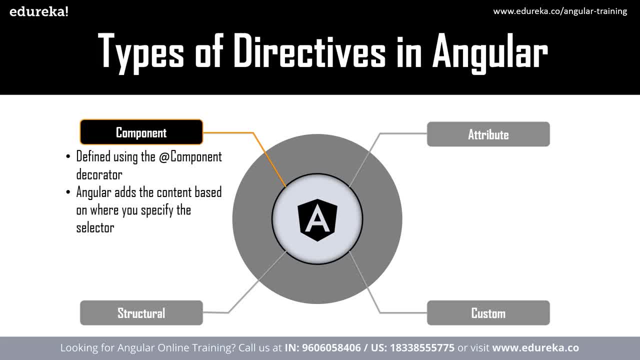 contents of your component at that particular position. As you all know, whenever a new Angular application is created, the root component or the app component will be created by Angular. When you open the app-componentts file, you will be able to see the selector of the app. 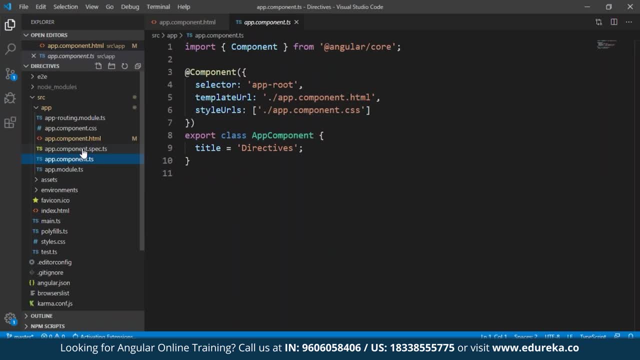 component or the root component. I have already created a project over here. In case you have any doubts on how to create an Angular project, check out the Angular 8 tutorial from Edureka. So, as you can see on the screen, the selector for the root component is present within the 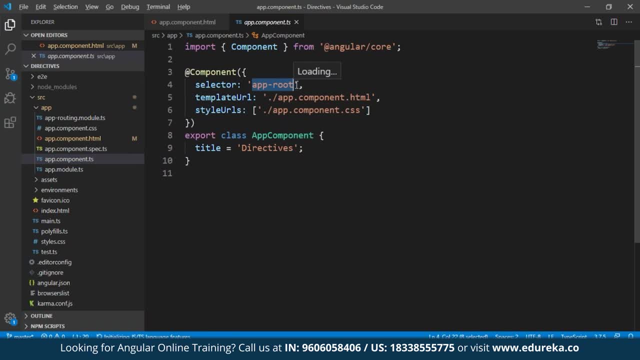 at-the-rate component decorator. This selector will be present in the indexhtml template by default. Okay, so now let me just open indexhtml file for you all to see this. So whenever you create a new component, Angular creates the required TypeScript file, the. 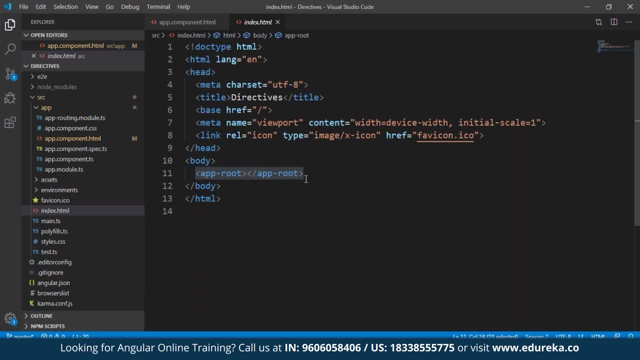 test file, the HTML file and the CSS file. The selector of the component will be present within the TypeScript file. So now let me just create a component in order to show this to you all. To create components in Angular, you need to make use of the ng-componenttxt component. 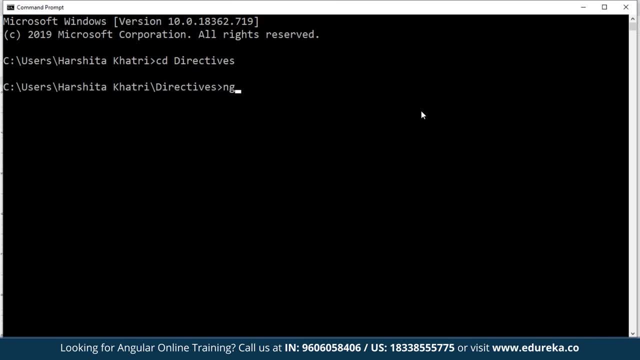 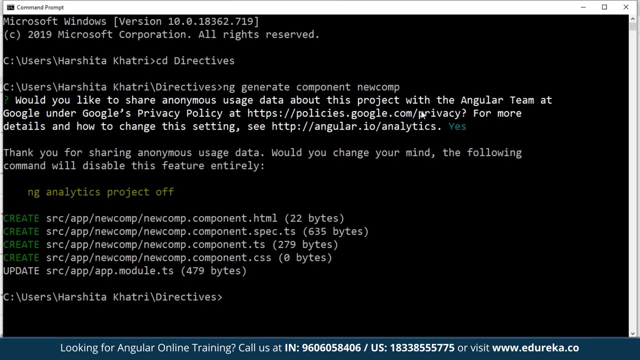 command. So I'll just open up the command prompt and I'll type ng- generate component. and you can give any name to this, so I'll just name it as newcomp. So I will just copy the selector and I will add it to the app-componenthtml file. 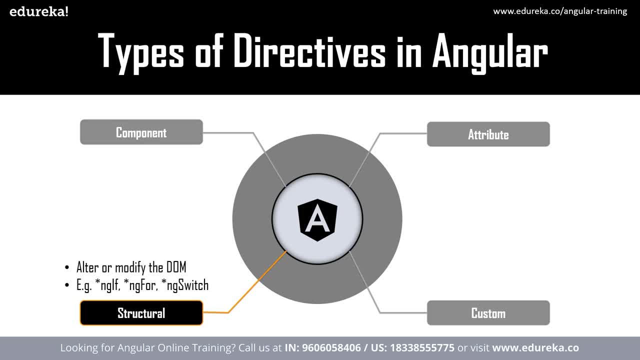 Okay, so now moving on towards the structural directives. in Angular, structural directives are used to alter or manipulate the DOM. This is done by either adding, changing or removing the elements. A single element can have only one structural directives. Some of the most common examples of structural directives are ng-for, ng-if and ng-switch. 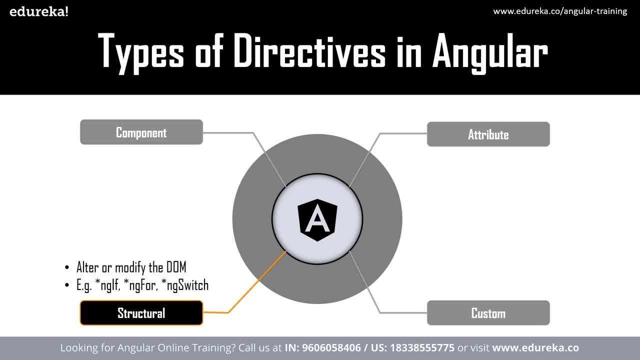 Before getting into the details of each of these, let me first tell you guys about the ng-template element of Angular. The ng-template element is used to render HTML in Angular, But this element is never visible directly. Therefore, before the views get rendered, Angular will not be visible. 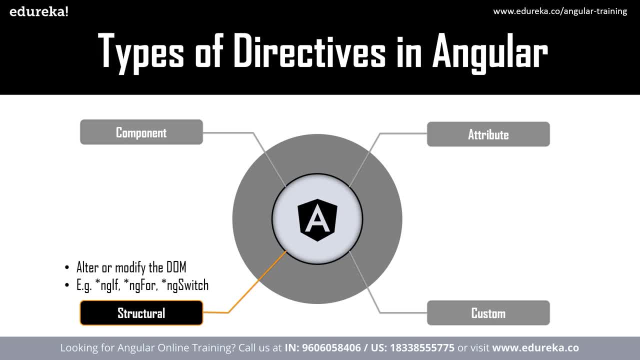 Therefore, before the views get rendered, Angular will not be visible. Angular will replace this ng-template element, along with its content, with a comment. If the view does not have any structural directive and you simply encase some elements in the ng-template element, those elements will disappear. 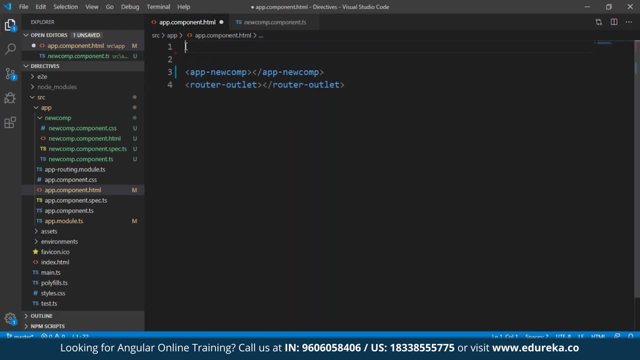 So let me just show you guys how this works. So what I'm going to do over here is just write welcome to Edureka and encase to within the ng-template tag. Okay, so just within the h2 tag I'll write welcome and within ng-template tag I'll write. 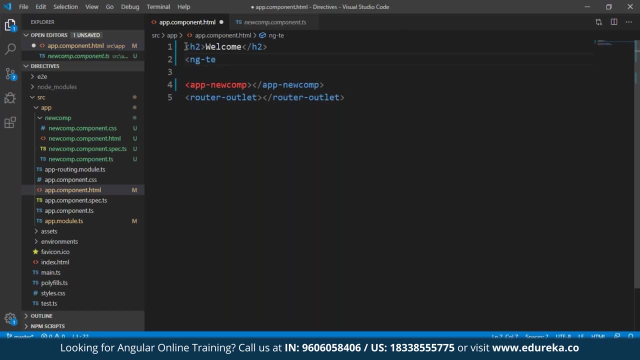 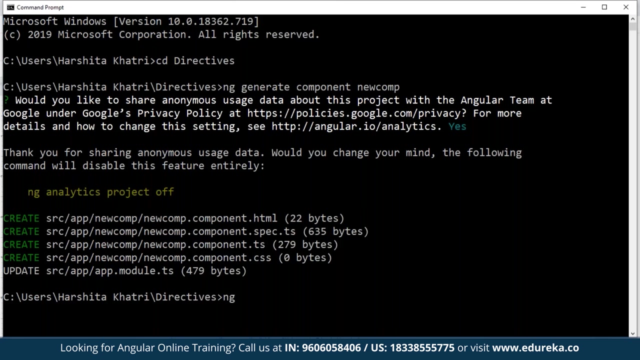 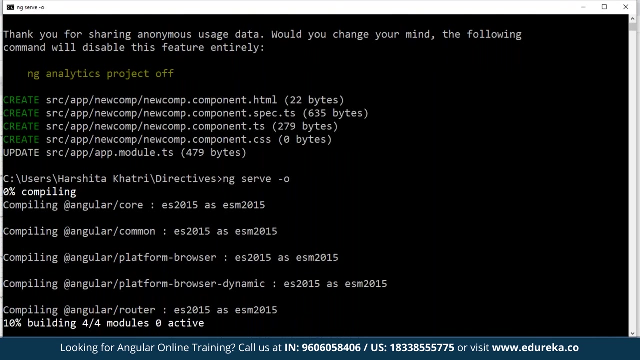 to And within an h2 tag again I'll write Edureka. So now I'm going to save this and type ng serve zyphn 0 in the command prompt. As you can see on the screen, the tool from welcome to Edureka is missing. 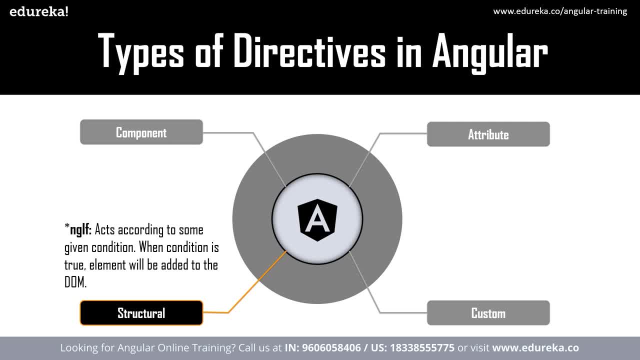 So let's paste that back on, Cool. So now let's move on and understand the working of ng-if, ng-for and ng-switch directives. One of the simplest structural directives is ng-if. This directive basically acts according to the given condition. 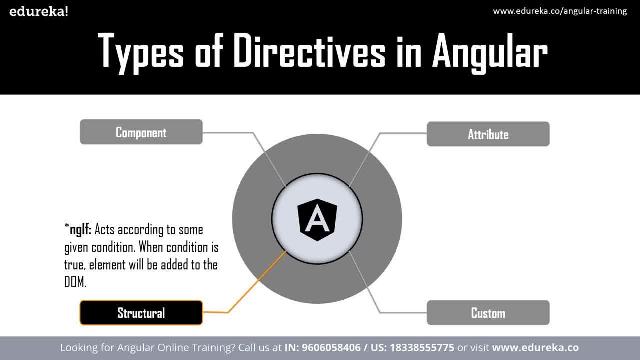 In case the condition is evaluated to true, a copy of the element will be added to the DOM. Otherwise, the HTML element will be removed. Structural directives are preceded by an asterisk symbol. You can write the ng-if directive by setting it to a string. 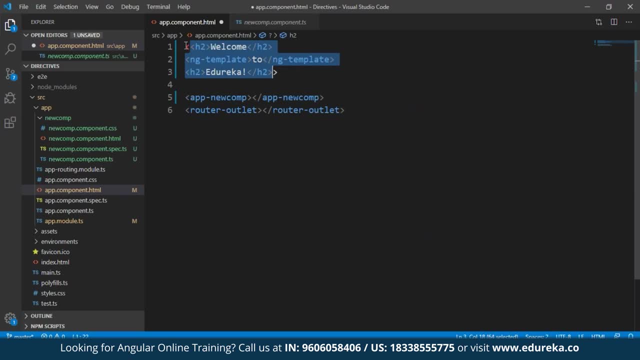 For example, if you want to print the name of some fruit, what I'm going to do is just open up a div tag and then I'll make use of star ng-if And I'll set this to a string that is fruit Class. over here will be name. 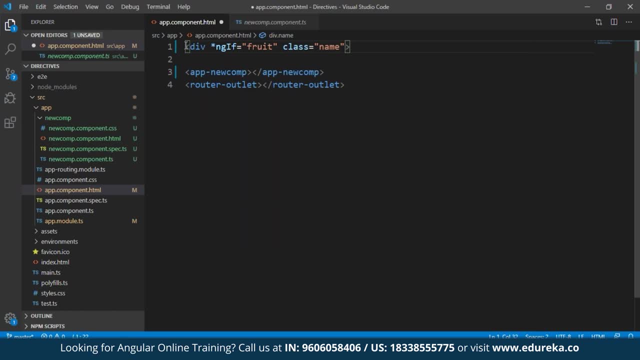 And since I want to print the name of the fruit, I'll just write fruitname within the interpolation brackets. So, as you can see, the star ng-if directive is set to a string And this string is called as a microsyntax. Microsyntax allows you to configure the directive in a friendly manner. 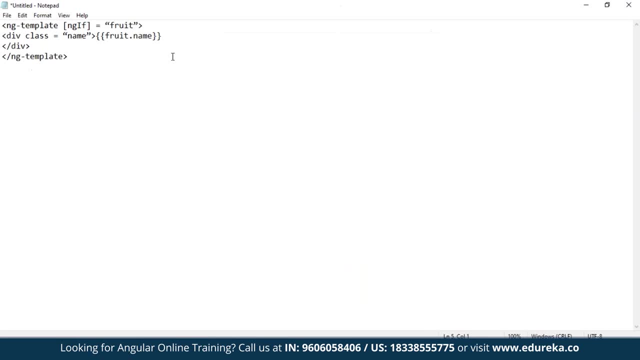 Angular internally converts this directive as follows. As you can see on the screen star ng-if gets moved by the ng-template element And the rest of the content, including the class, is moved within the ng-template element itself. I will create a small demo project and explain both ng-if and ng-for after we understand. 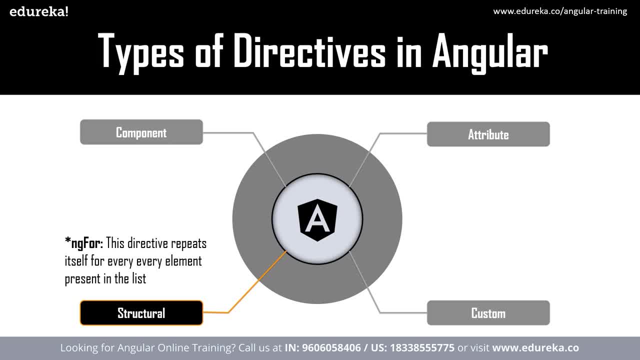 the working of ng-for. Okay, so ng-for- The ng-for directive- is called as a repeater directive And this directive is called as a repeater directive And this string is called as a micro-syntax. This directive will repeat for every element present in the given list. 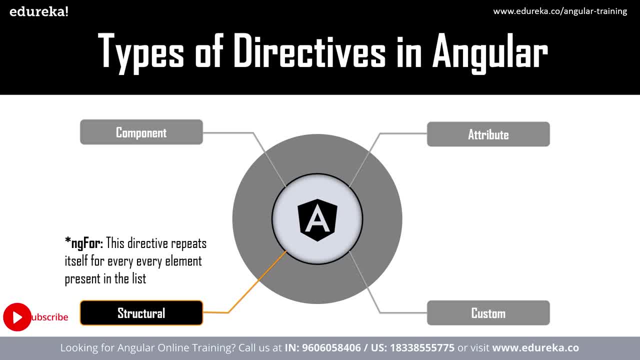 Just like we saw for ng-if, ng-for also gets transformed by Angular from the asterisk syntax to the ng-template element. Star ng-for is much complicated compared to star ng-if because it has many more dependencies, which can be both mandatory and optional dependencies. 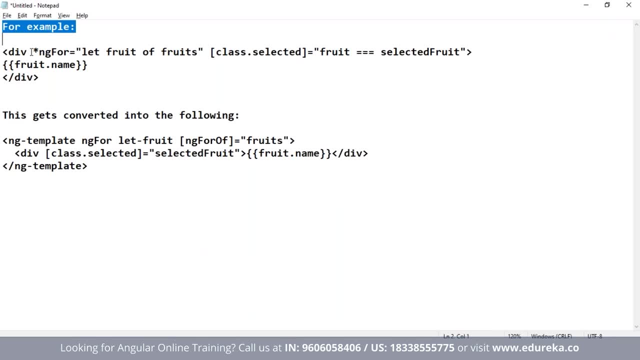 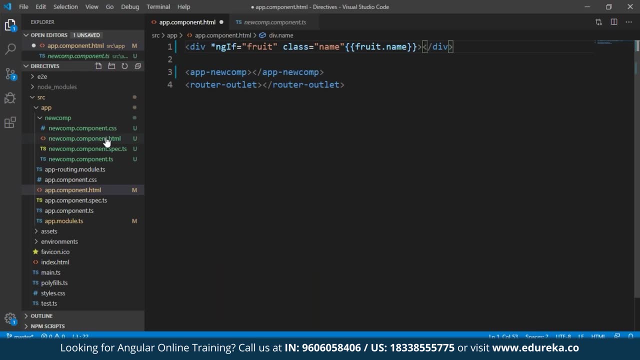 So in this example, the ng-for class requires a looping variable, that is the fruit and the list, that is the fruits list. To show you, guys, an example of both star ng-if and star ng-for, I will create a small Angular application. 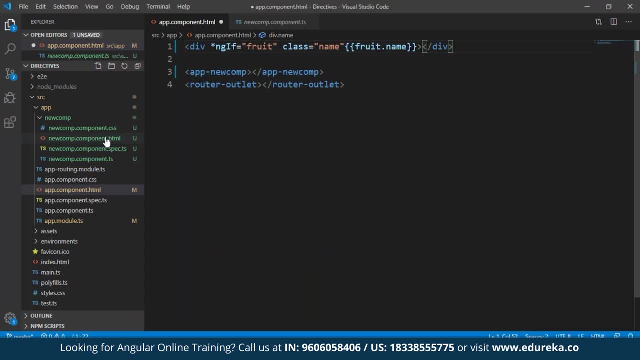 Okay, within this application, I will create a new file called as the fruitts file. So what I'm going to do is just right click on the app folder and type in the name of the file, that is, fruitts. Now, within this file, I will create an interface. 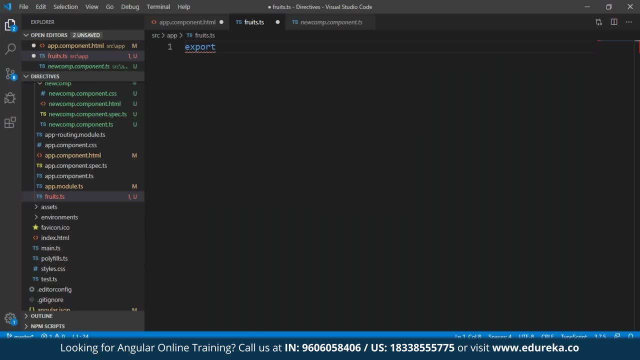 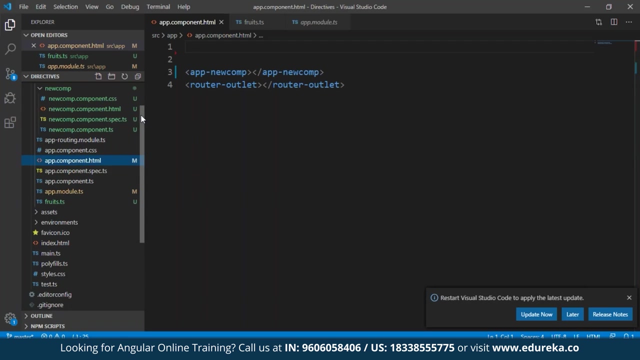 Okay, so export interface and the name of the interface, which is fruit. Now, within this I'll have two properties, that is, the id and the name. So id will be number and name will be of type string. So once this is done, I will create another fruit listts file that will hold the list. 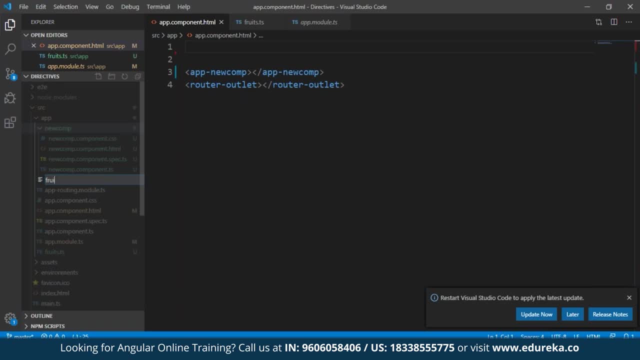 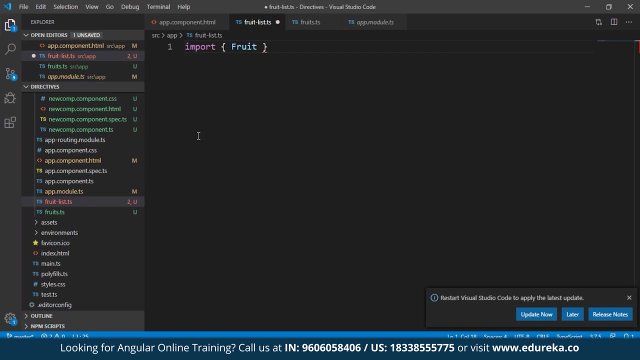 of fruits. The first thing that I will have to do over here is import the fruit interface from the fruitsts file. So I just import fruitts, Okay, From fruits. Then I will create the list of fruits, So the first fruit will have id number one. 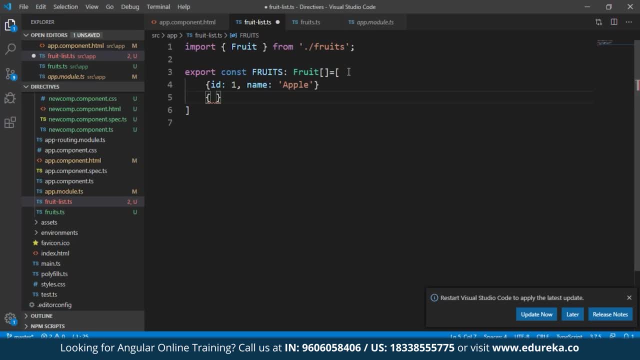 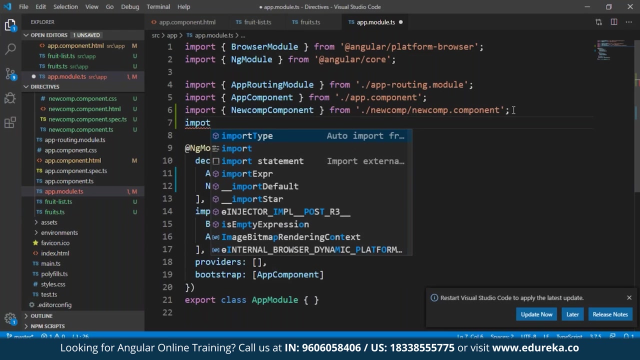 And the name will be apple. The second fruit will have id two And the name will be anything say, for example, mango. Next I will open the app modulets file and then I'll add the forms module to it. So import forms module from angular forms. 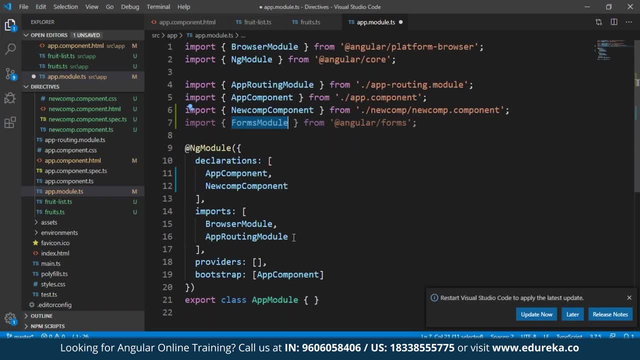 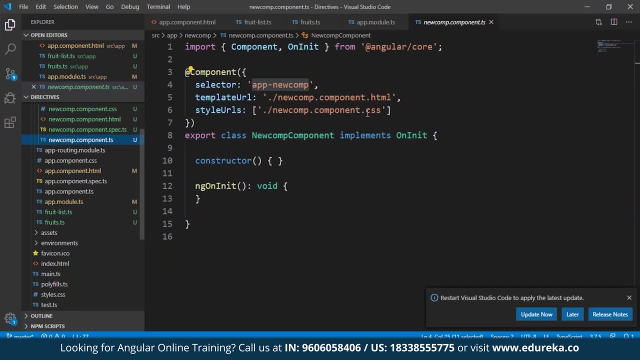 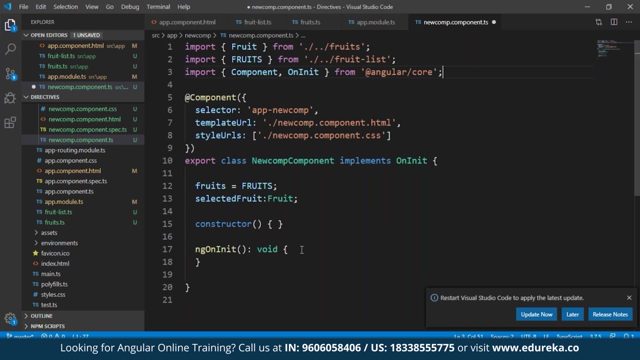 I should also include it within imports, so I'll just import forms module. Okay, So I'll open the new compts file, add two new properties, that is, fruits and the selected fruit. Next I'll create a new function, that is the onSelect function, which will return the details. 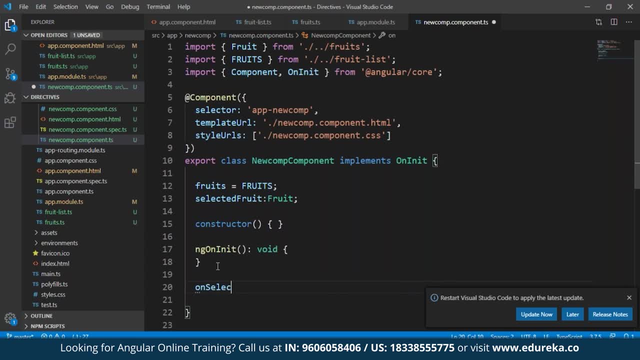 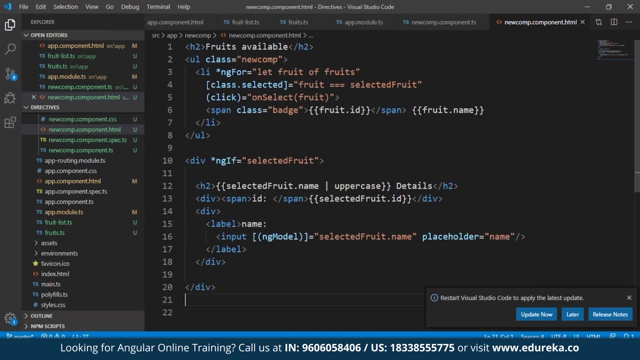 of the selected fruit. So onSelect fruit which is of type fruit And return type will be void Thisselected fruit equals fruit. Okay, so now I'll open the new compcomponenthtml file. Over here I'm going to paste the code that I have already written for ng-if and ng-for. 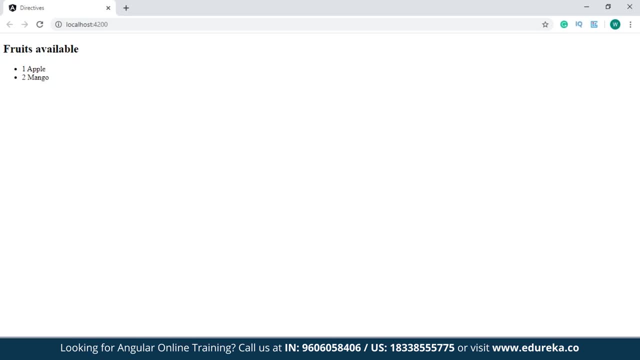 Okay, so I'll save this and I'll get back to my development server. Okay so, as you can see on the screen, I have the list of fruits that are available. When I click on any of these fruits, you'll be able to see the details of them. 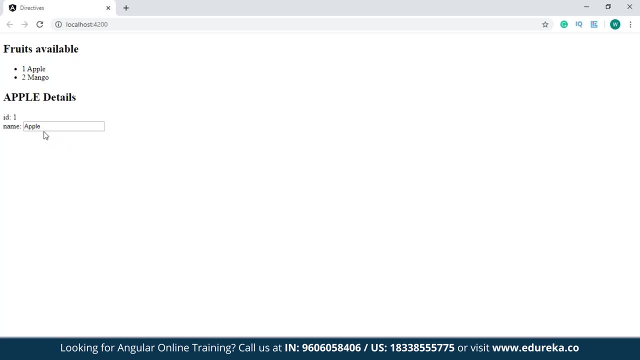 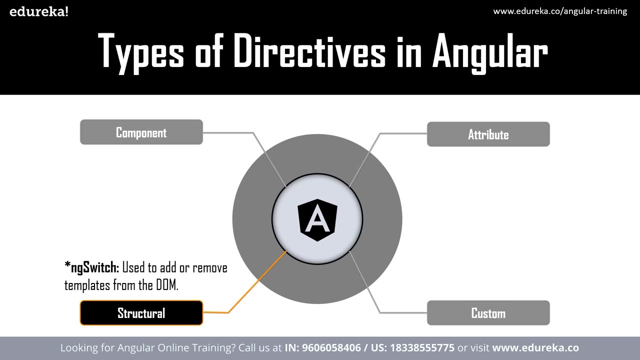 So I hope you guys have understood today. The next structural directive that we'll learn is the star ng-switch directive. The star ng-switch directive is used to add or remove templates from the DOM. This is done by specifying an expression that is to be matched. 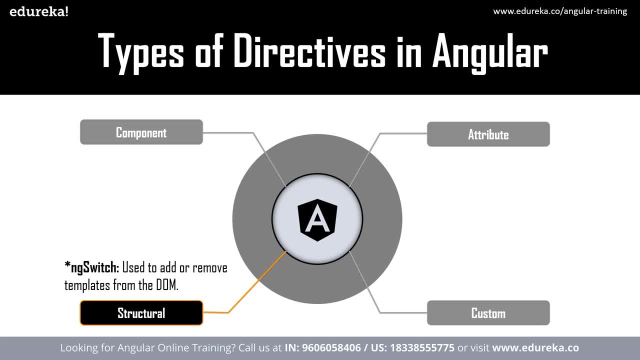 The star ng-if directive is actually a set of collaborating directives. The expression that is required to be matched will be specified using the ng-switch case directive within the same container element. So what I'm going to do is just paste the code that I have already written. 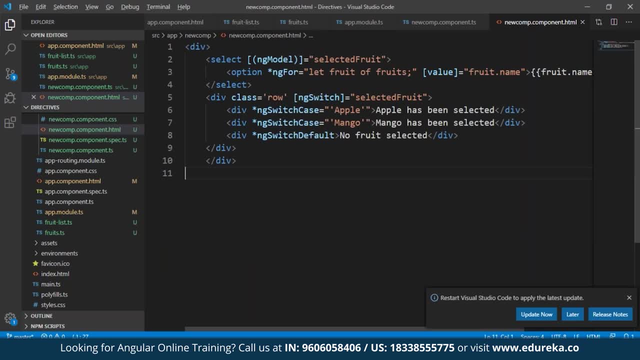 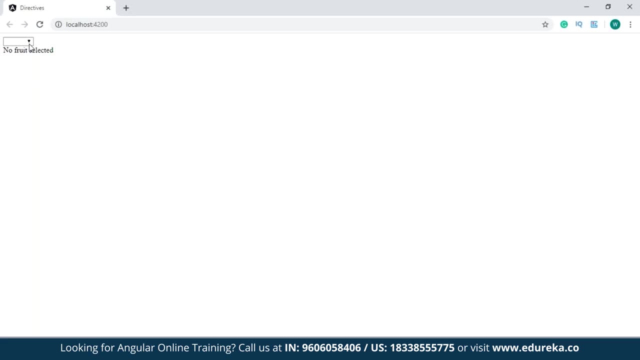 This code will produce the list of fruits within the drop-down list and I will be able to select any of them. Okay, so I'll just save this and I'll get back to my development server. Okay, so, as you can see on the screen, I have a drop-down list and a message saying no fruits. 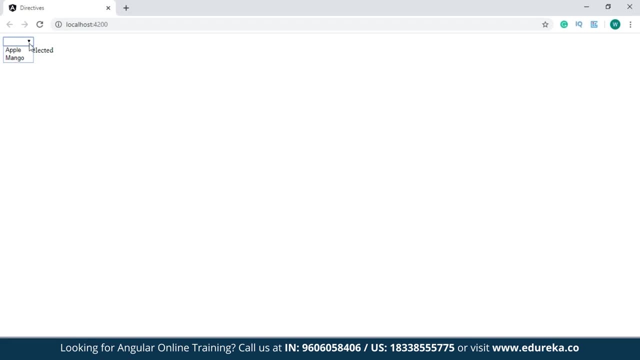 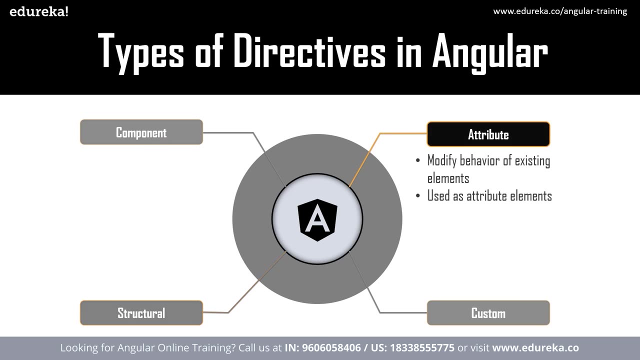 selected. When I click on any of these, I will get the corresponding message instead of no fruits selected, which is the default case message. Okay, so I hope you guys have understood till here. Now, moving on towards attribute directives: Input directives are used to modify the behavior or appearance of some existing element component. 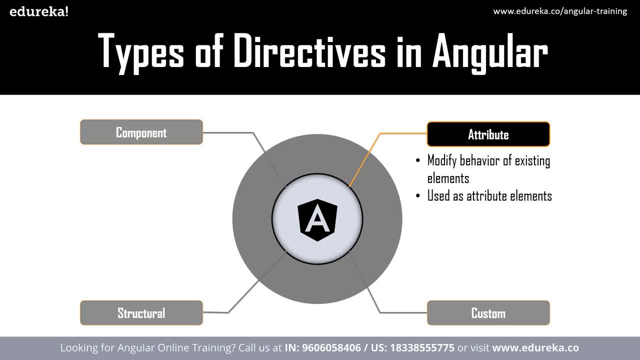 or some other directives. As the name suggests, these directives are utilized as attributes of elements within templates and they resemble the HTML attributes. One of the most common examples is the ng-model directive. This directive is used for two-way data binding. It is commonly used to modify the behavior of an existing element. that is usually the 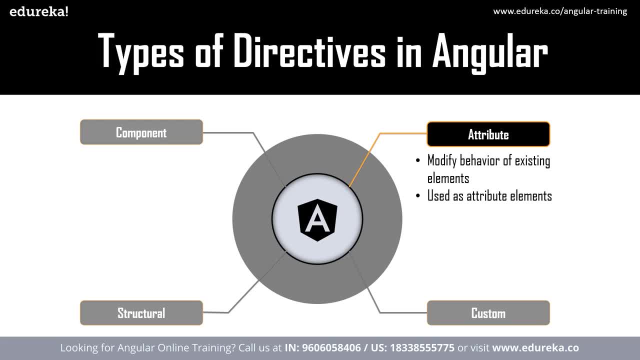 input element. ng-model sets the input element's display value property and it will also be used to change events that take place. For instance, consider the ng-model directive used in the previous example. Okay, so, as you can see on the screen, I've made use of the ng-model directive and this 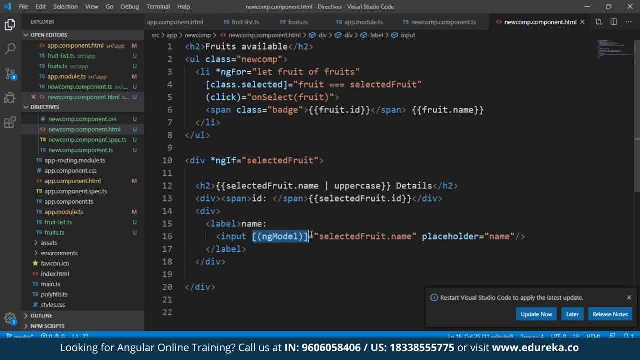 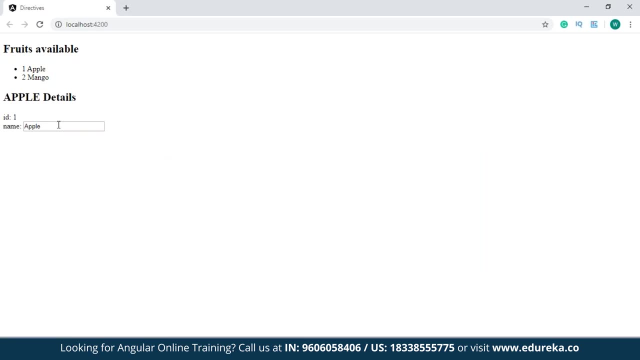 directive is used within the input tag. So what basically happens over here is: in case I make changes to the name of the fruit on the views, it will get reflected in the models as well. So let me just get back to my development server. 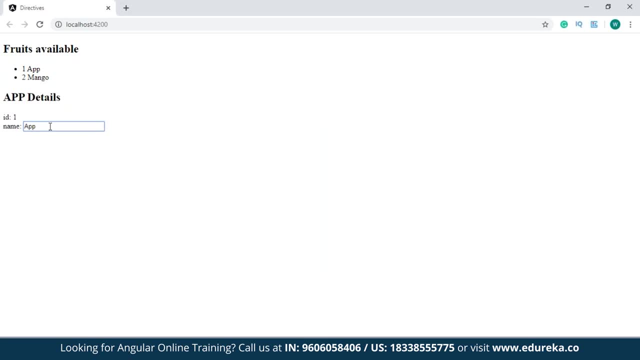 Okay. so what I'm going to do over here is try to change the name of apple, Okay. So, as you can see, When I make changes to the name of apple, the corresponding change is reflected in the name of the fruit present in the models as well. 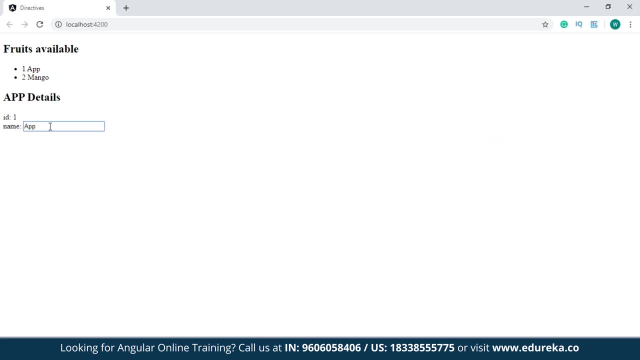 This is an example of two-way data binding. Here the models are modified using the views. The ng-model directive is a part of form control module. The form control module is used to keep a track of validation status, the value and the user interaction in order to keep the models in sync with the views. 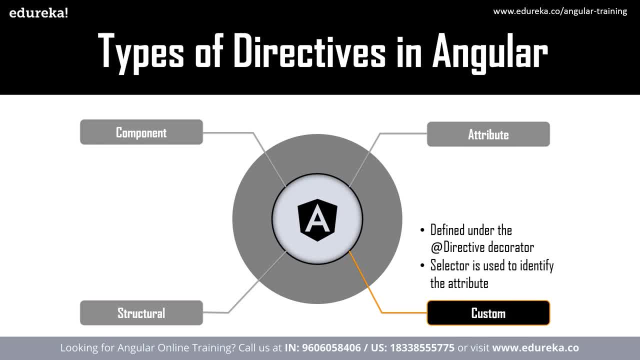 So now, moving on towards the custom attribute directives, The minimum requirement for an attribute directive is a class with the at-the-rate directive. So let's go ahead and do that. Let's create a class called ng-generate-directive-decorator. 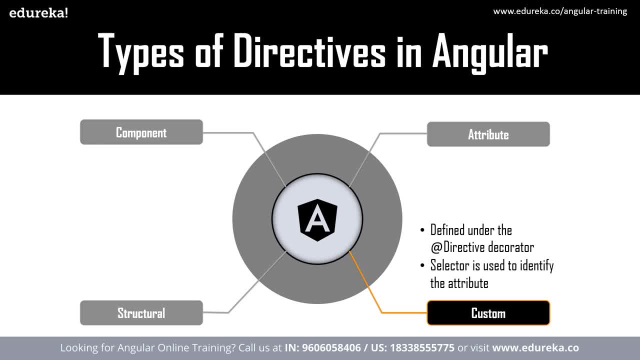 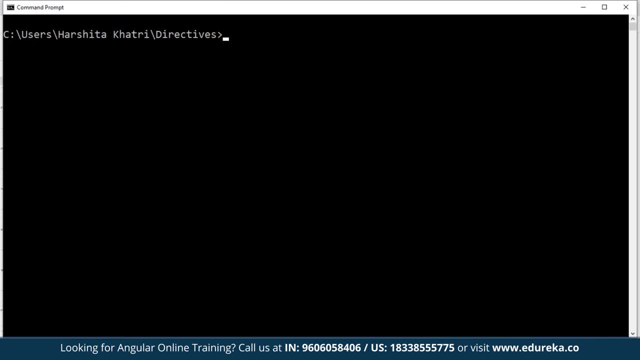 This class contains the selector that will identify the attribute. To create this directive class using the Angular CLI, you'll just have to type in the command ng generate directive, followed by the name of the directive. So what I'm going to do is just open up the command prompt and over here I'll type ng. 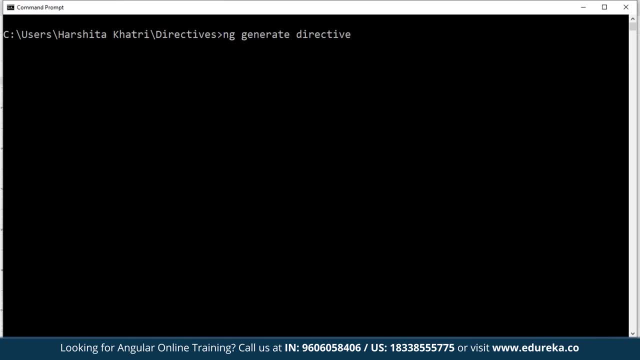 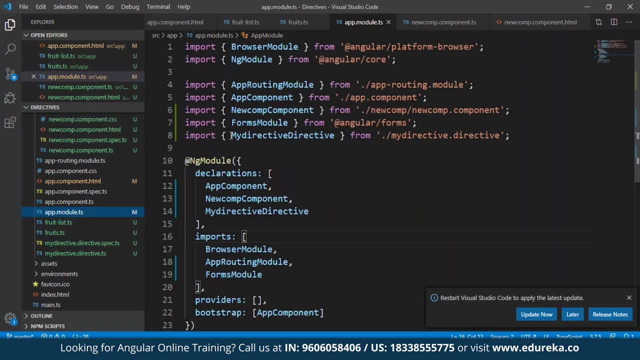 generate directive- my directive. So this will create two files, That is, the directivets file and the directivedirectivedecorator. These are the typescript and the test files respectively. The directives that you create should be declared within the modules, just like how it is done. 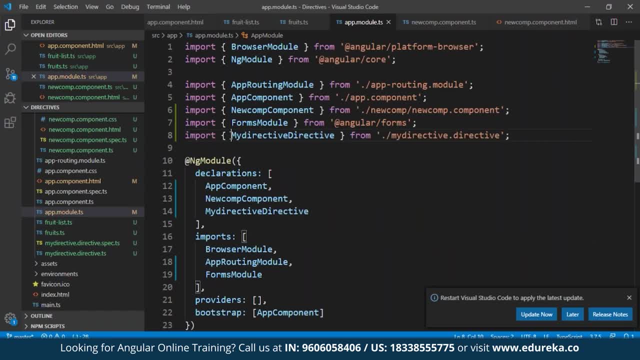 for components. Okay, so what I'm going to do is just open up the app-modulets file to show this to you guys. Okay, so, as you can see, the directive that I've just created has been auto imported. This is due to the auto import extension that I've added. 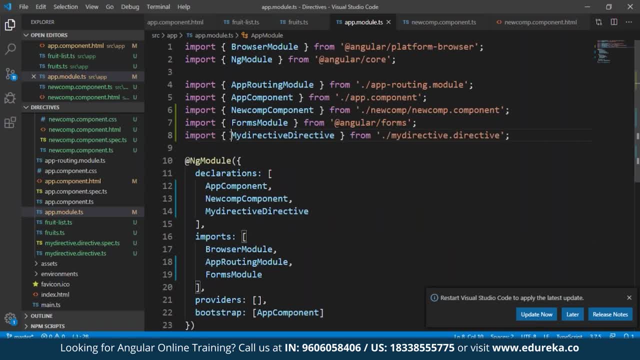 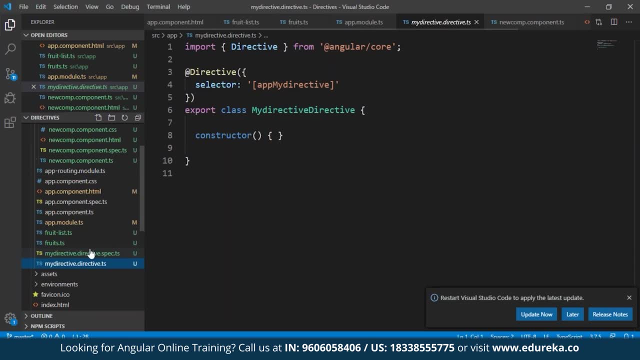 In case you do not have this extension, you will have to manually declare it. I'll just open the my-directivets file. The at-the-rate directive should be declared within the modules, just like how it is done for components. The at-the-rate directive decorator consists of a single configuration property that specifies: 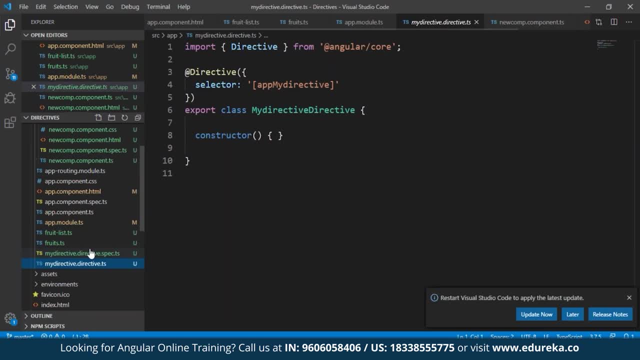 this directive's CSS attribute selector. In this case it's app-my-directive. The square brackets are used to make it an attribute selector. Whenever some element is found to have app-my-directive attribute in the templates, Angular will apply the logic of this directive to that element. 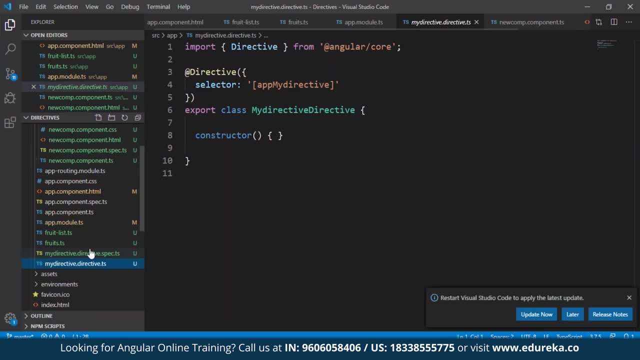 The first letter of the attribute directive is capitalized to avoid conflict with standard HTML attributes. Not just this, It also avoids conflict with the names of third party attributes. The first letter of the attribute directive is capitalized to avoid conflict with standard HTML attributes. Not just this: 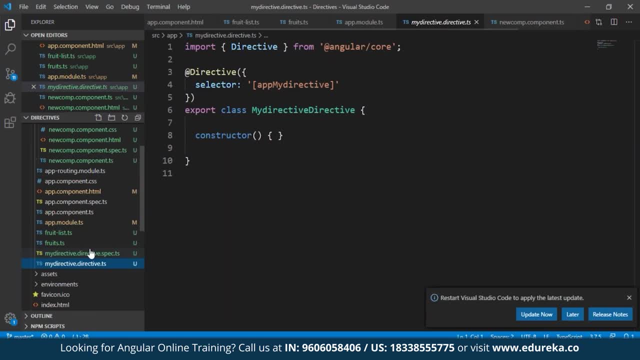 It also avoids conflict with the names of third party attributes. The app prefix is added by the Angular CLI. Below the at-the-rate directive metadata is the collector class called as my-directivedirective. This class will hold the logic for this directive. You can also export my-directivedirective to make it accessible. 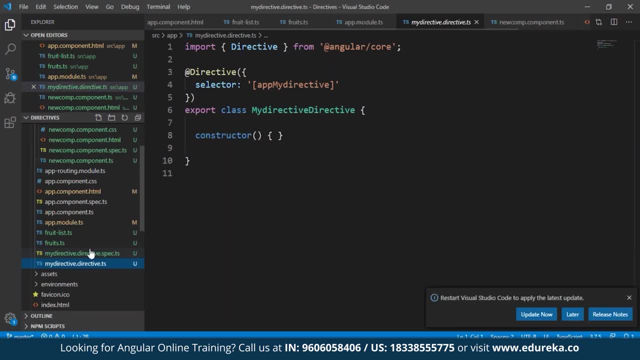 So, in order to modify this file, I'll make use of the element ref, which is a wrapper around some native elements inside the views present in Angular core library. Here the element ref wrapper is specified within the constructor In order to inject a reference to the host DOM element. that is the element to which 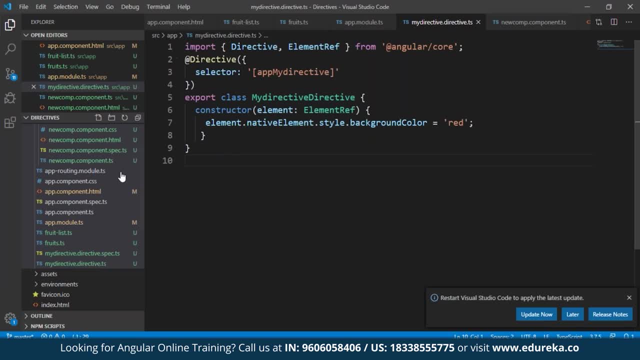 the app. my-directive has been applied, So I already have a code over here. I'll just paste it and I'll save this. To demonstrate how this works, I'll just open up the app-componenthtml file And over here I'll open a div tag. 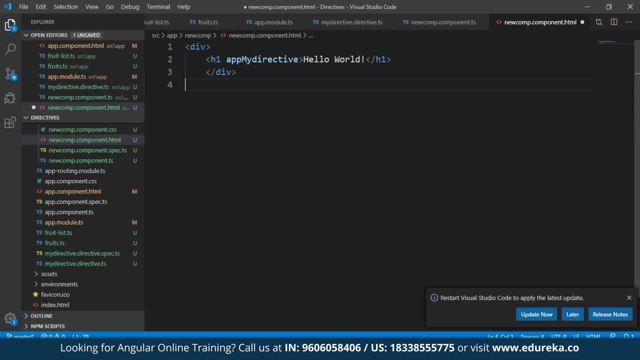 Within that, I'll open an h1 tag, write app my-directive, and within this I'll just write hello world. Okay, I'll just save this. So basically, in this case, I'll just write hello world. In this code, the app my-directive attribute is detected by Angular on the host h1 tag. 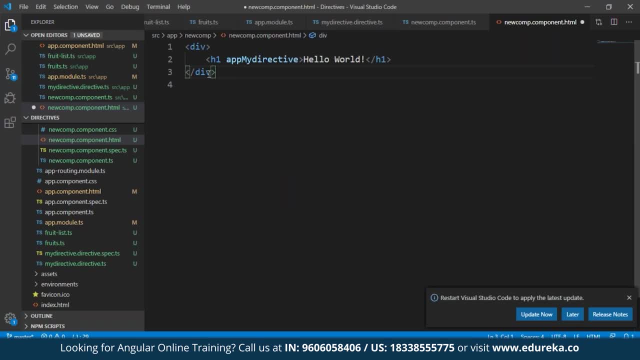 Then Angular creates an instance of my-directive directive class. It then injects a reference of h1 element into the directive's constructor, which sets the h1 element's background style to red. Okay, so I'll just save this. So now I'll just type in ng serve and I'll open the development server. 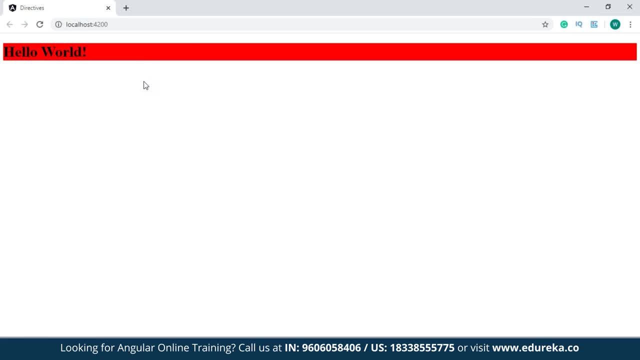 Okay. so, as you can see on the screen, hello world has been highlighted with a red color. In this instance, I've specified the element's background color to be red. You can further configure the CSS according to your preferences. So this brings us to the end of this session. 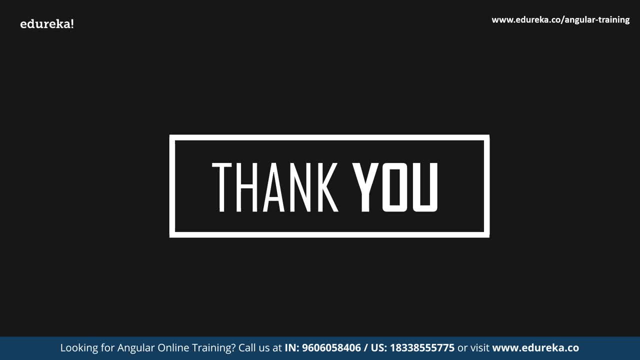 I hope you guys have enjoyed and learned something new. In case you have any doubts or queries, please do let me know in the comments section and I will revert to you at the earliest. We'll be back with more and more exciting sessions, but till then, goodbye and take. 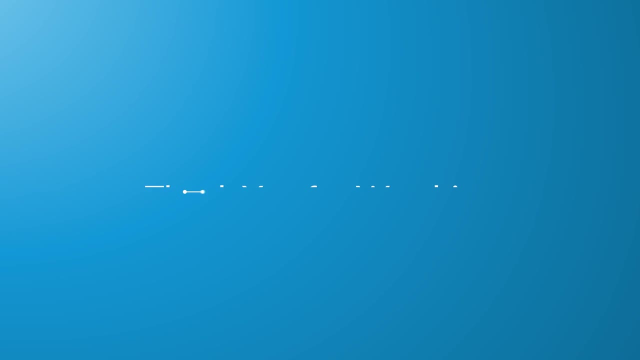 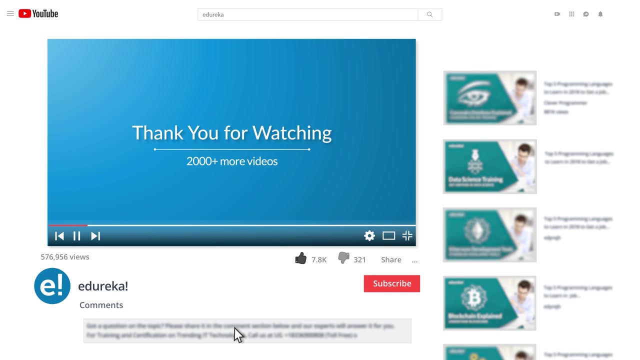 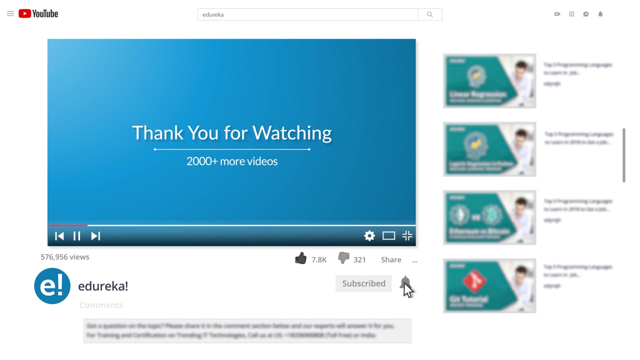 care. Do look out for more videos in our playlist and subscribe to Edureka channel to learn more Happy learning.